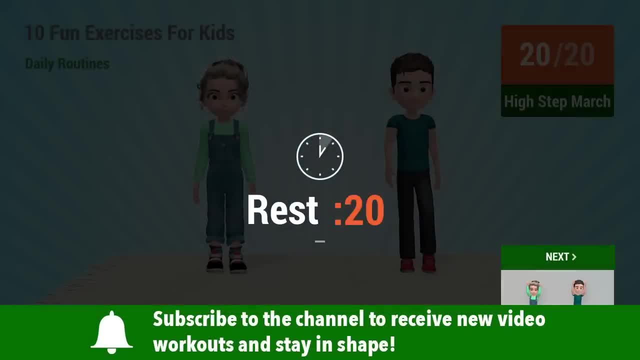 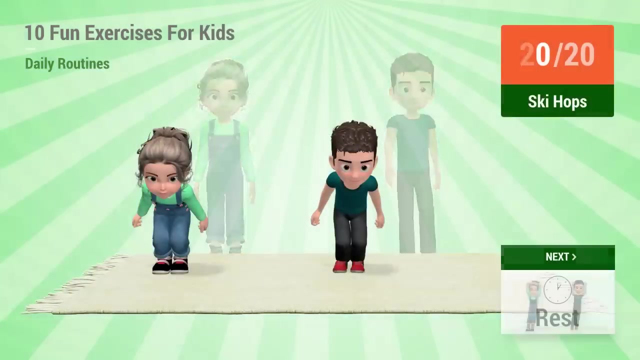 19,, 20,, 21,, 22,, 23,, 24,, 25,, 26,, 27,, 28,, 29,, 30., 19,, 20, rest time. Up next ski hops in 5,, 4,, 3,, 2,, 1, go. 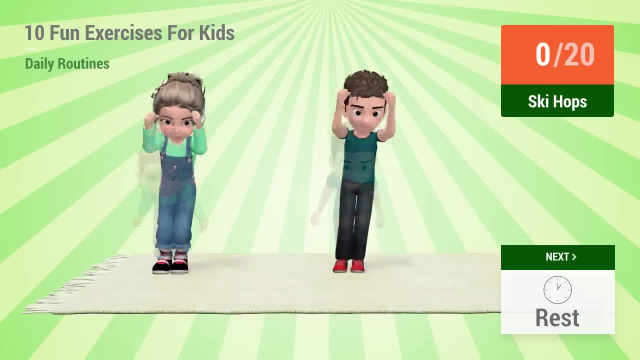 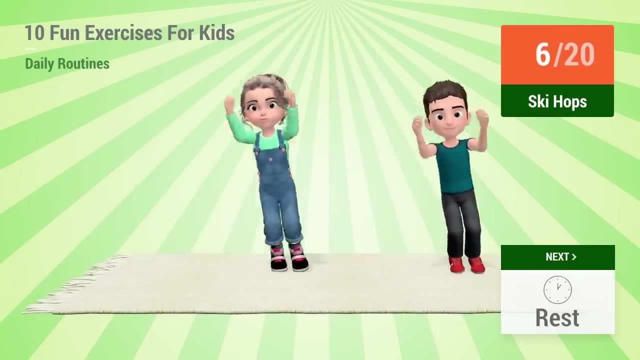 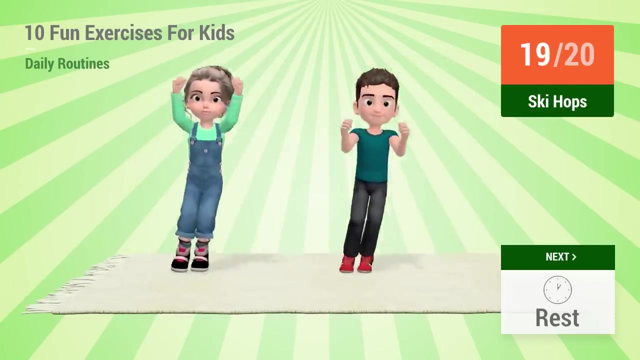 1,, 2,, 3,, 4,, 5,, 6,, 7,, 8,, 9,, 10,, 11,, 12,, 13,, 14,, 15,, 16,, 17,, 18,, 19,, 20,, 21,, 22,, 23,, 24,, 25,, 26,, 27,, 28,, 29,, 30. 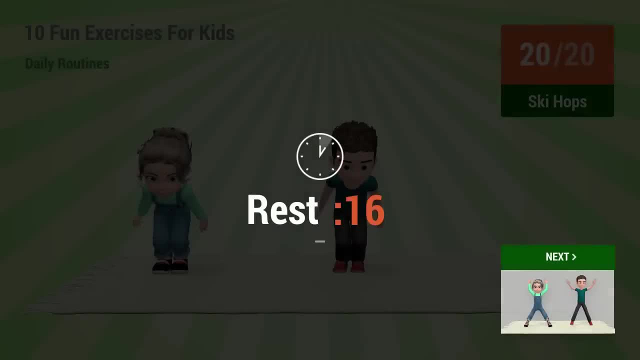 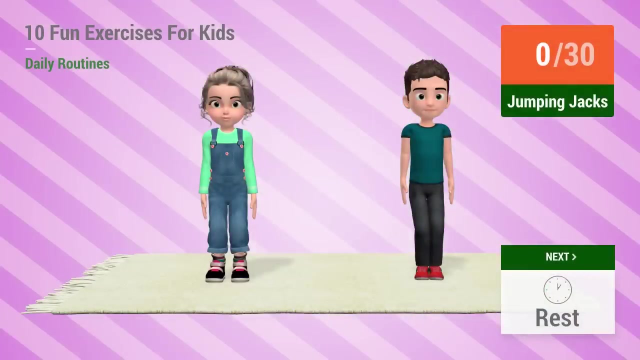 Rest time. Up next, high knee jacks in 5,, 4,, 3,, 2, 1, go 1, 2, 3,, 4,, 5,, 6,, 7,, 8,, 9,, 10,, 11,, 12,, 13,, 18,, 19,, 20,, 21,, 22,, 23,, 24,, 25,, 26,, 27,, 28,, 30. 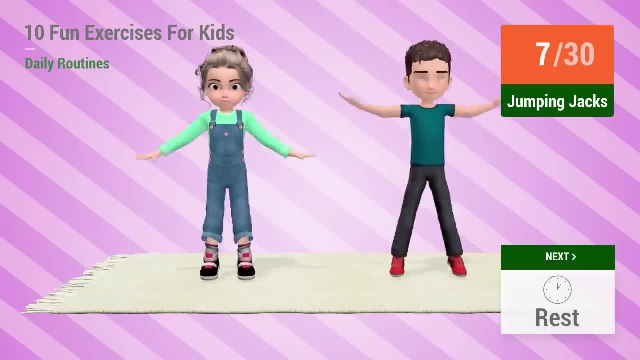 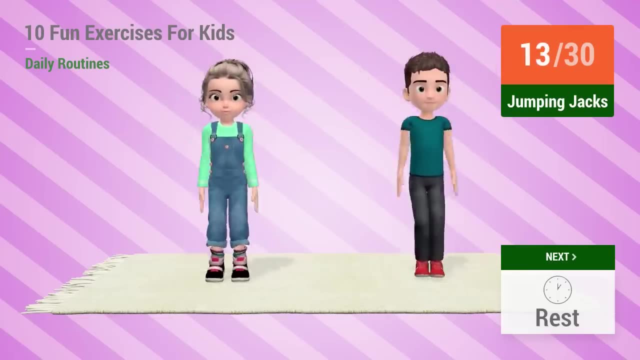 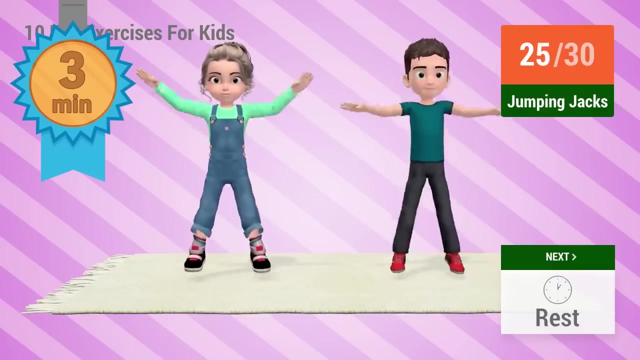 Rest time: 1,, 2,, 3,, 4,, 5,, 6,, 7,, 8,, 9,, 10,, 11,, 12,, 13,, 14,, 15,, 16,, 17,, 18,, 19,, 20,, 21,, 22,, 23,, 24,, 25,, 26,, 27,, 28,, 29,, 30. Rest time: 1,, 2,, 3,, 4,, 5,, 6,, 7,, 8,, 9,, 10,, 11,, 12,, 23,, 24,, 25,, 26,, 27,, 28,, 30.. 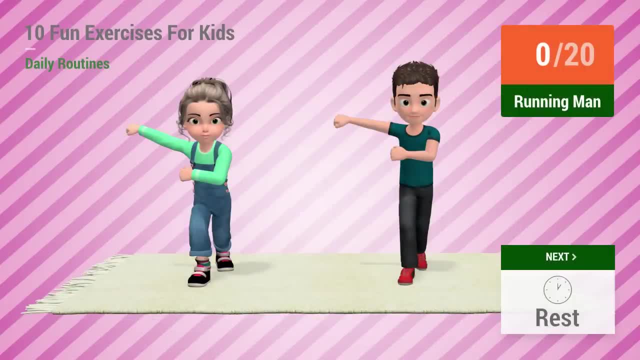 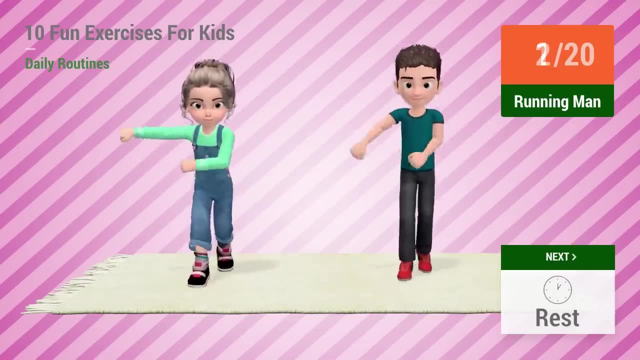 Up next running man in 5,, 4,, 3,, 2,, 1, go 1,, 2,, 3,, 4,, 5,, 6,, 7,, 8,, 9,, 10,, 11,, 12,, 13,, 14,, 15,, 16,, 17,, 18,, 19,, 20.. 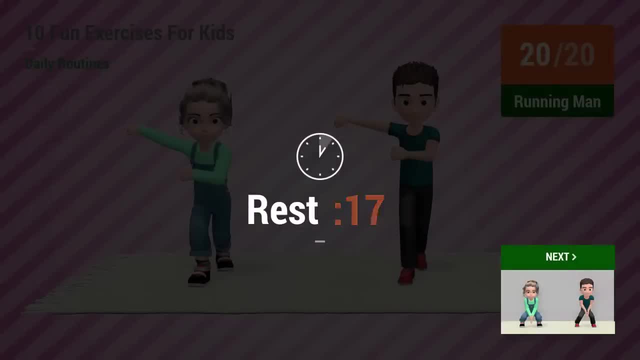 Rest time: 1,, 2,, 3,, 4,, 5,, 6,, 7,, 8,, 9,, 10,, 11,, 12,, 13,, 18,, 19, 20.. 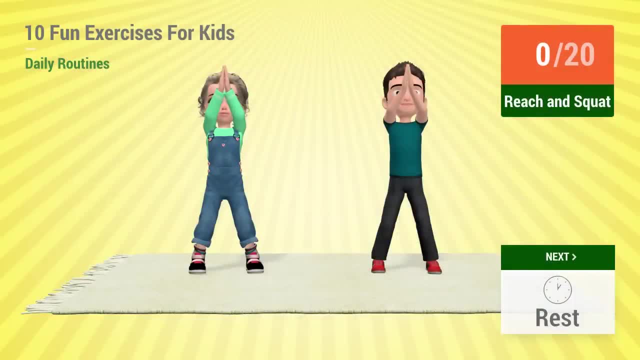 Up next reach and squat in 5,, 4,, 3,, 2,, 1, go 1,, 2,, 3,, 4.. 1,, 2,, 3,, 4,, 5,, 6,, 7,, 8,, 9,, 10,, 11,, 12,, 13,, 14,, 15,, 16,, 17,, 18,, 19, 20.. 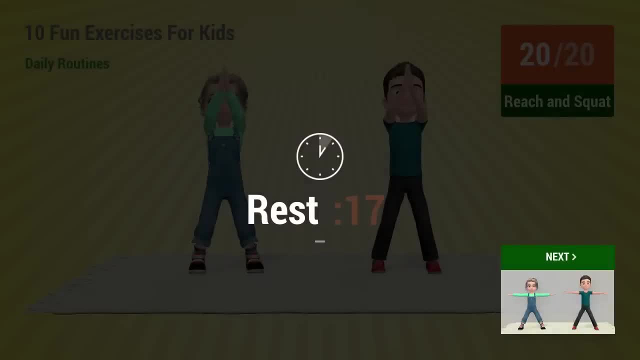 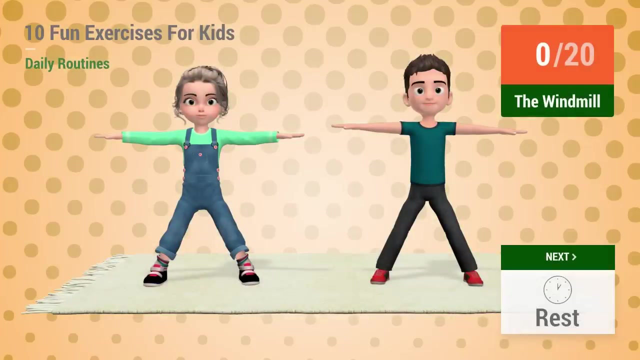 Rest time. Up next the windmill in 5,, 4,, 3,, 2,, 1, go 1,, 2,, 3,, 4,, 5,, 6,, 7,, 8,, 9,, 10,, 11,, 12,, 13,, 14,. 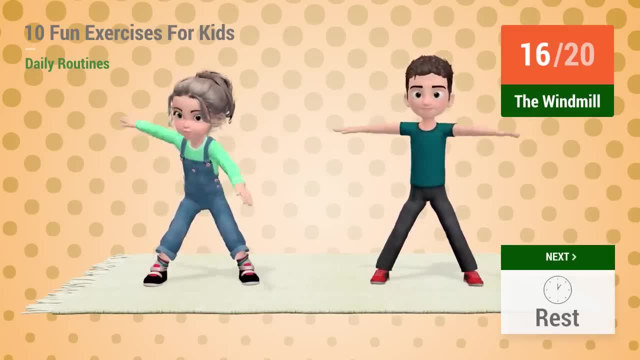 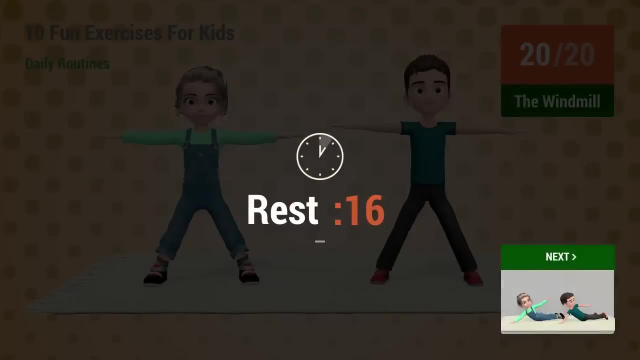 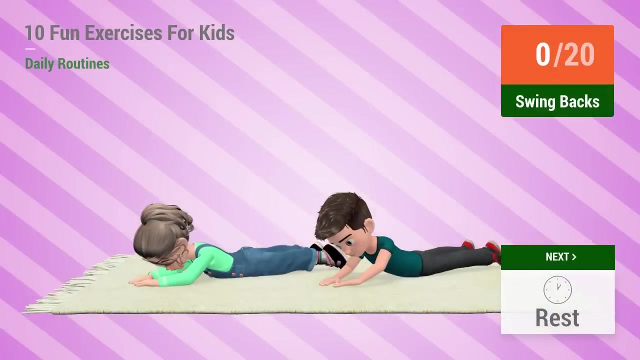 15,, 16,, 17,, 18,, 19,, 20, rest time. Up next swing backs in: 5,, 4,, 3,, 2, 1, go 1,, 2,, 3,, 4,, 5,, 6,, 7,, 8,, 9,, 10,. 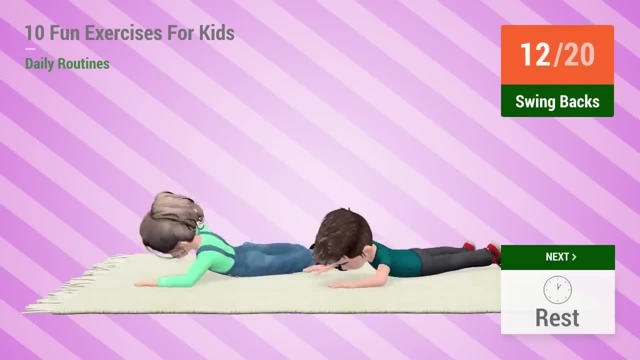 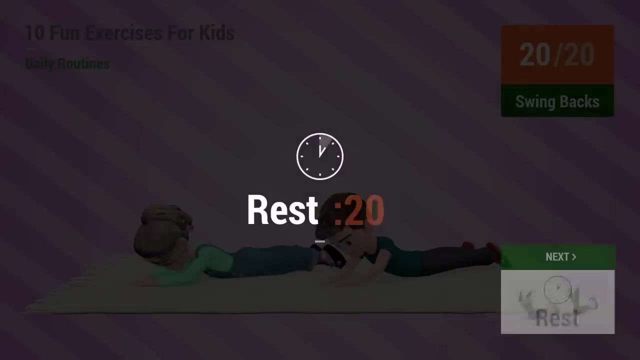 11,, 12,, 13,, 14,, 15,, 16,, 17,, 18,, 19,, 20, rest time. 1,, 2,, 3,, 4,, 5,, 6,, 7,, 8,, 9,, 10,, 11,, 12,, 13,, 14,, 15,, 16,, 17,, 18,, 19,, 20, rest time. 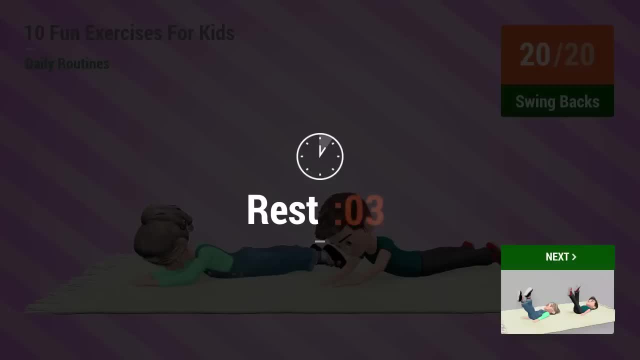 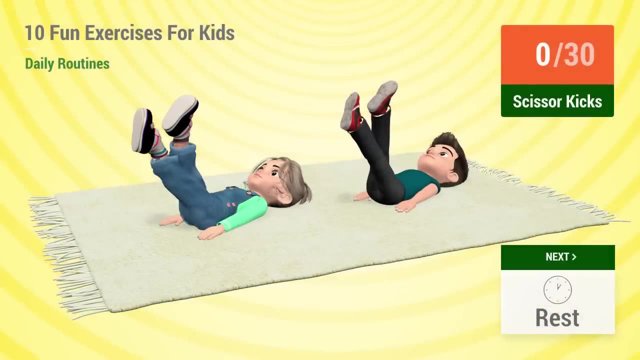 Up next scissor kicks in: 5,, 4,, 3,, 2,, 1, go 1,, 2,, 3,, 4,, 5,, 6,, 7,, 8,, 9,, 10,, 11,, 12,, 13,, 14,, 15,, 16,, 18,, 19,, 20, rest time. 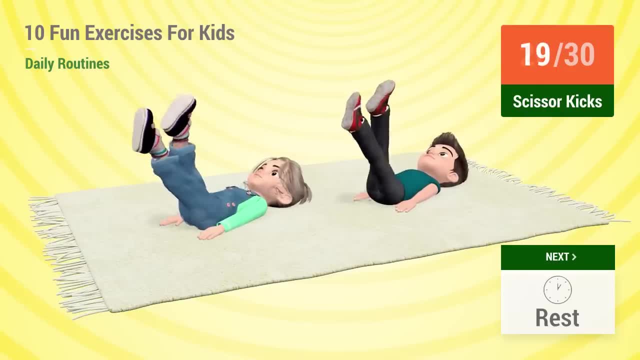 1,, 2,, 3,, 4,, 5,, 6,, 7,, 8,, 9,, 10,, 11,, 12,, 13,, 14,, 15,, 16,, 17,, 18,, 19,, 20,, 21,, 22,, 23,, 24,, 25,, 26,, 27,, 28,, 29,, 30, rest time. 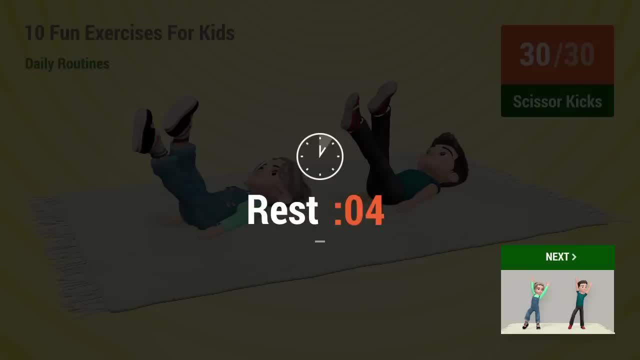 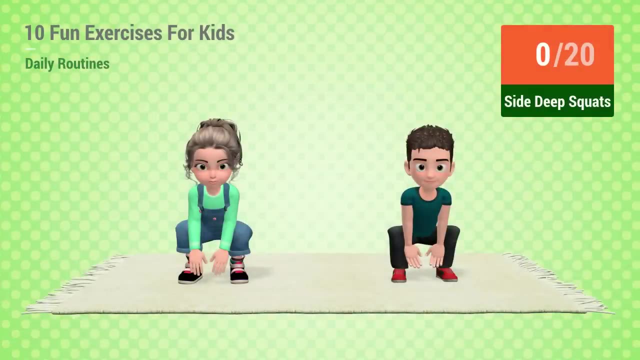 1,, 2,, 3,, 4,, 5,, 6,, 7,, 8,, 9,, 10,, 11,, 12,, 13,, 18,, 19,, 20, rest time.